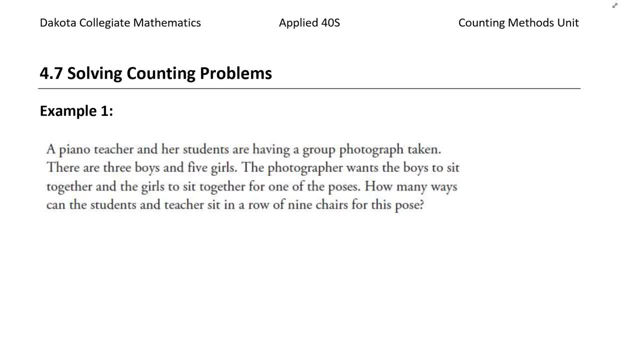 In this lesson we're going to look at solving counting problems, And all that means is that we're taking everything that we learned in this unit and putting it together. So your responsibility now is to look at each question that you are faced with, like on a test, on an exam, on an assignment, and decide: is this fundamental counting principle, Is this a permutation, Is it a combination? Do I do an exponent here? 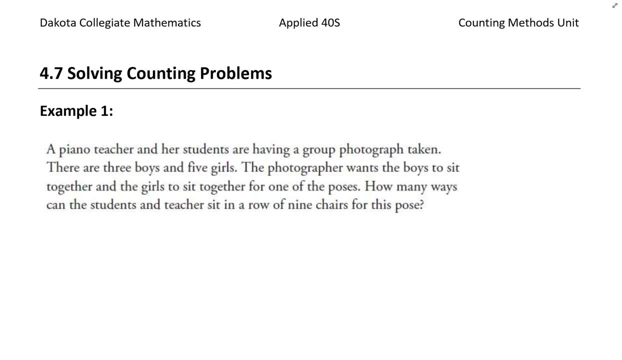 Right? Is this a factorial type problem? What is it that I'm doing? So, always identify. what is it that you're given, Right? What is known, What is unknown? What are you trying to solve for? And does order matter? Does order not matter, Right? Those are all the questions you're going to ask yourself. as you're going to go through these types of questions, We're going to do a couple together and then we'll do more in class. So it says, a piano teacher and her students are having a group photograph. 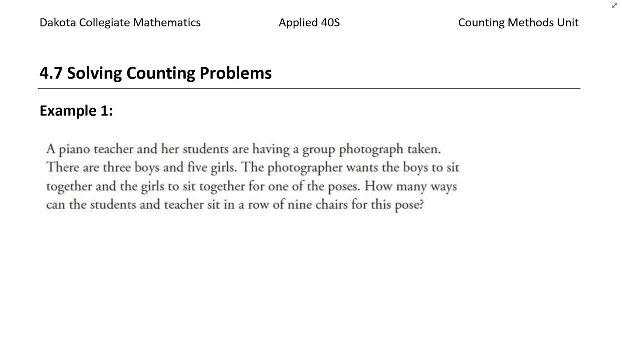 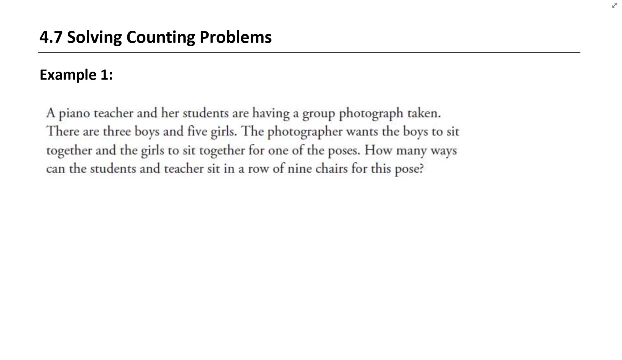 There are three boys and five girls. The photographer wants the boys to sit together and the girls to sit together for one of the poses. How many ways can the students and teachers sit in a row of nine chairs for this pose? So I was like, whenever we get these types of questions, like the red car question, draw out the dashes, right, Let's draw that out. So we've got how many people here total? 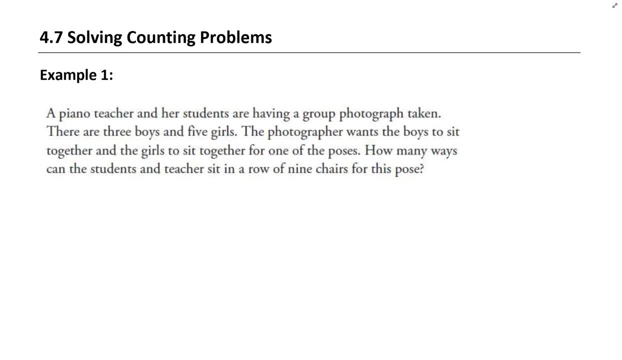 It says there are three boys and five girls, And then you've also got the teacher, So all right. so there we go. That will accommodate the row of nine chairs for this pose. Now the boys are sitting together Right, So let's do the three boys here. 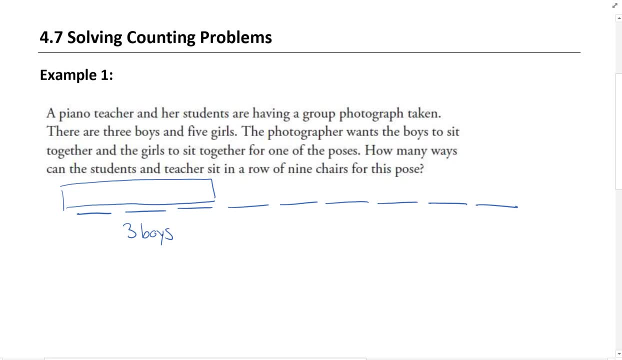 And then we've got the five girls, And then finally we've got the one teacher. Now the three boys themselves can sit in the first, second or third position, and then they can have all the different arrangements in those three positions. 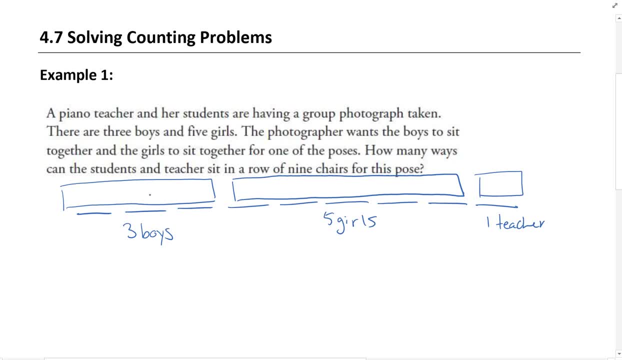 So that would give me three times, two times one or three factorial Right? So if we just use the boys here in those three positions, any of the three could sit here Once the person, once the one kid sits down, then any two, And once that person sits down, then that's the last one, Right? That would give us three factorial. 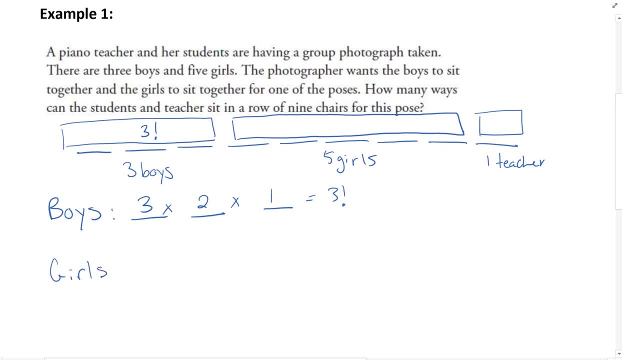 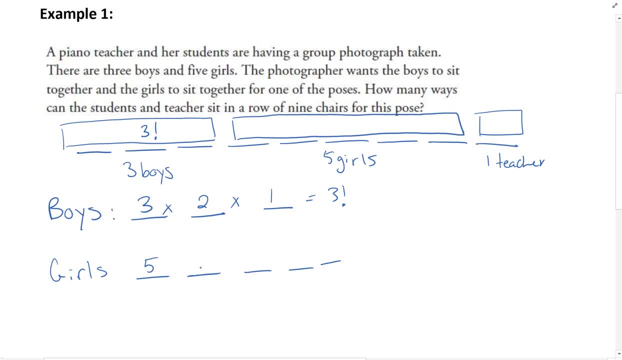 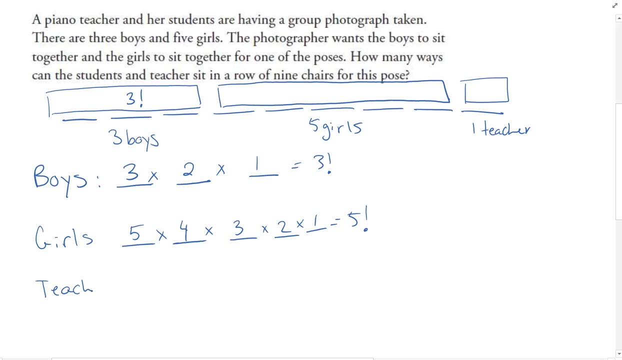 Yeah, Yeah, Yeah, And that would be the same as five factorial. And then the teacher. Well, there's only one teacher, So there's only one way for the teacher to sit there. So this would be five factorial and this would be one, And at that point you kind of feel like you're done right. 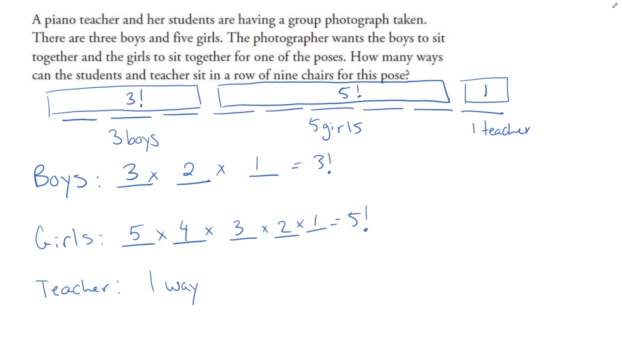 Yeah, I've done all the math, I've done all the work and that's fine. However, these three students that are sitting here can be moved to this position or can be moved to that position, Right? So there's more than just that position for three factorial. 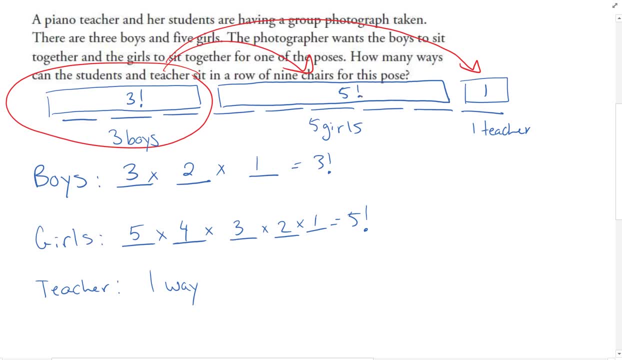 The three factorial can sit where it is, or it can move in the middle position or at the end. And then, if you look at the five girls, they can stay where they are or they can go here, or they can go here. 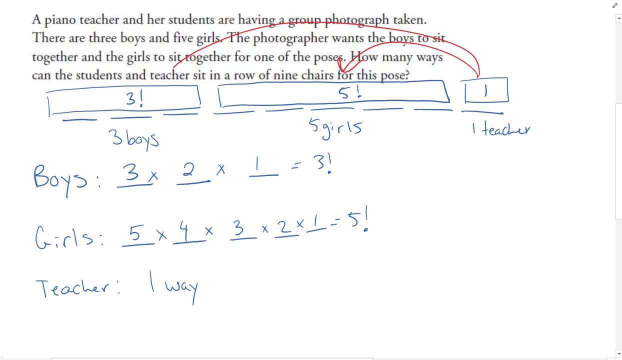 Right, And then the teacher can sit in the middle between the boys, and girls can sit at this end, or the teacher can sit at the end that they already are sitting. So how do we accommodate that? Okay, Okay, So, because we're treating this kind of like three different. 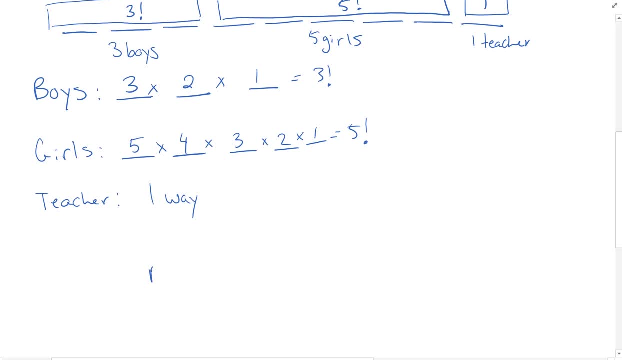 objects. right, If I screen this down. we've got the boys in one position, the girls in another position and the teacher in another position, But they can all move between their positions. So if I have those three objects to choose from, I would have either the boys or the girls or the teacher there. 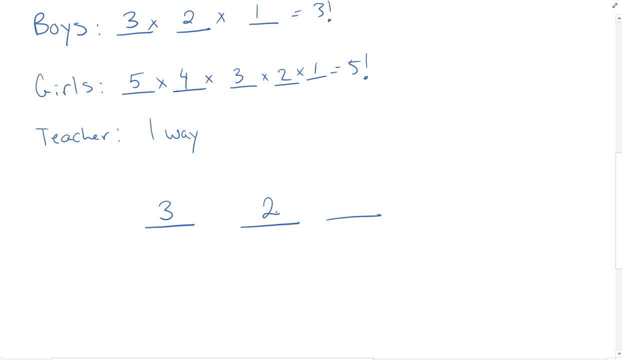 Once one of those groups are placed, then I have the other two groups that can be placed there in the lounge And then I have the last group to be placed there. So this is accommodating the various groups that could sit in those positions, which would be three factorial. 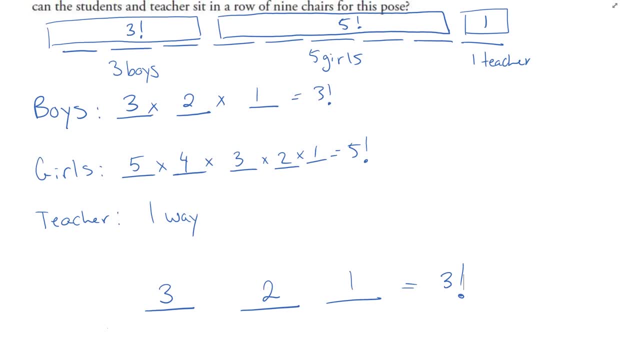 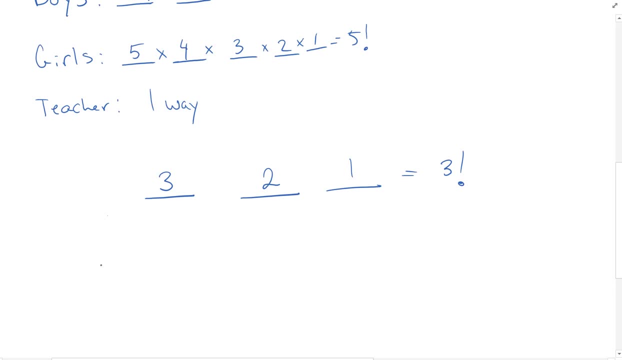 But it's not just the groups, It's also within the groups. The three boys are three factorial, the five girls are five factorial and the teacher's one. So the answer here for the number of arrangements would be exactly what I was just saying. 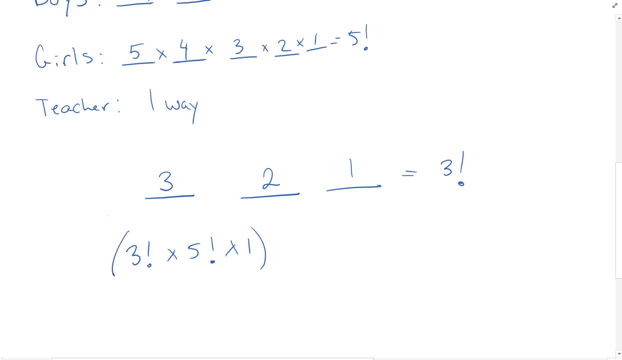 Three factorial times five factorial times one, Which is what we're seeing Up top, But then all of that is going to be multiplied by the three factorial So and we can move those groups around to give us 4,320 weeks to arrange that group. 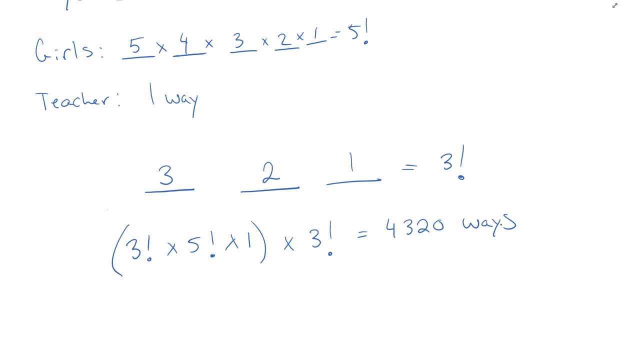 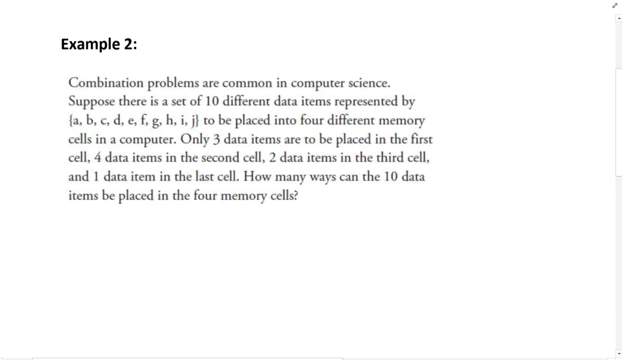 Okay, so you might want to go back and look that over again, But we get those types of questions often. We'll do some more practice in class. Okay, let's take a look at the next one. Okay, so these types of questions come up and I'm going to explain how to recognize that it's this type of question. 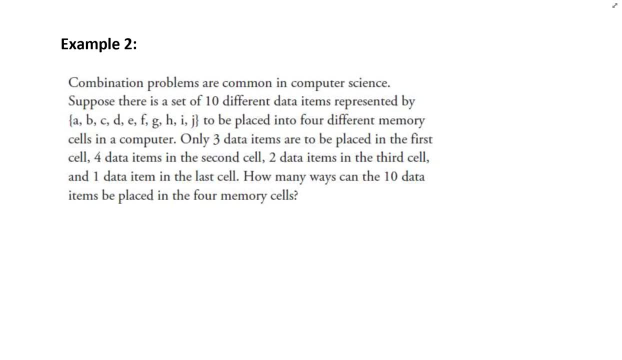 There's always going to be variations. but I'll explain how we can see that It says combination problems are common in computer science. Suppose there's a set of 10 different data items represented by the letters A through J. Now those items are to be placed in four different memory cells on a computer. 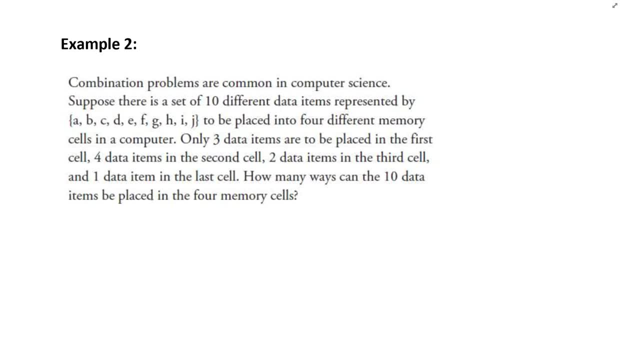 Okay, Only three data items are to be placed in the first cell, four in the second, two in the third and one data item in the last cell. How many different ways can 10 data items be placed in the four memory cells? 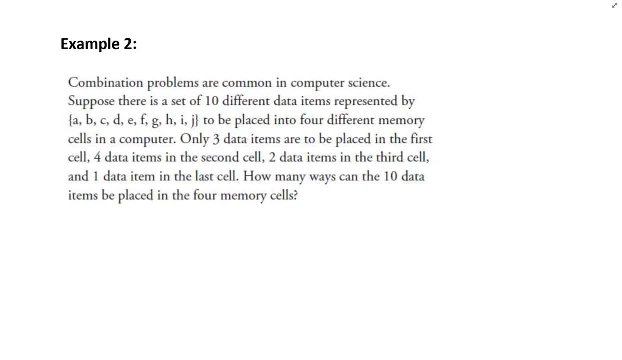 Now, if the fact that we're dealing with computer stuff is completely throwing you, I don't understand what they're talking about. You can think of this as in people being placed in cars. You can think about like to get a ride. You can think about this in terms of students being placed in classrooms to work on things. 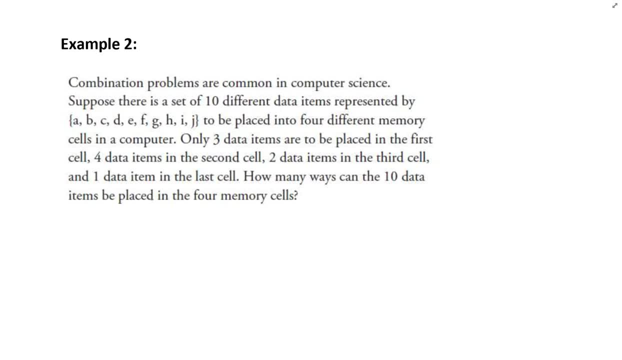 You can think about this as maybe filling boxes with donuts, Like whatever you want to do, you have so much stuff, right? 10 different items of stuff. In this case it's data items and it's to be placed in different spots. 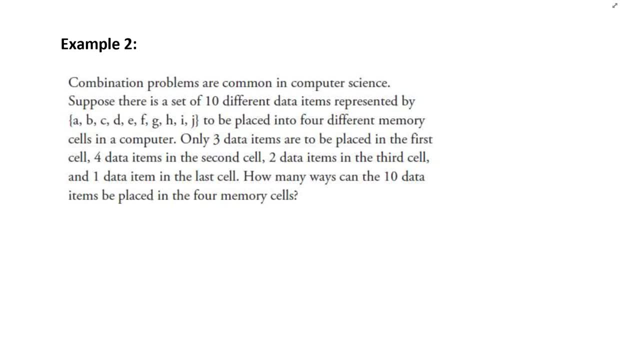 Now you've got to think: once you've placed something in a spot, you're not taking it out of its spot anymore. It's already there, Okay. So, thinking about this, we've got A through J right, All those different items. 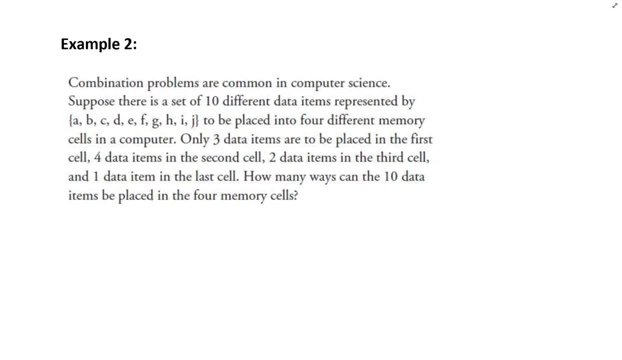 And we want to know how many ways can the 10 data items be placed in four memory cells? So we're going to look at the number of ways that we can put them into cell 1, the number of ways in cell 2,, the number of ways in cell 3, and the number of ways in cell 4.. 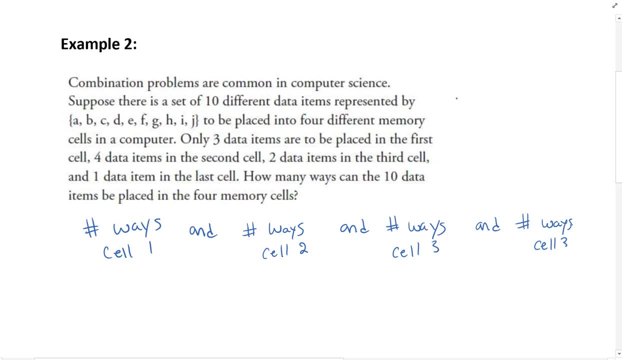 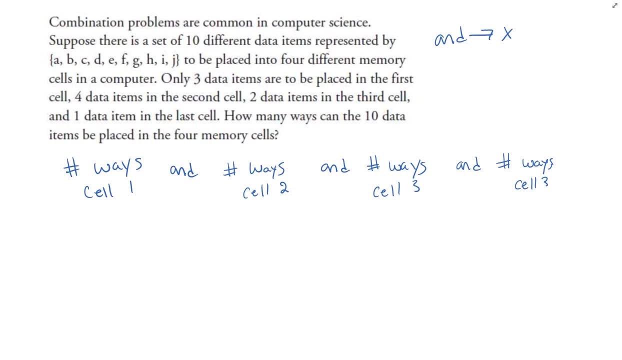 Now you can see I wrote and in between all of them, And remember, and And means multiply, because all of that has to hold true. Okay, Not or, but, and It's not different cases. All of these things are happening for that problem to be solved. 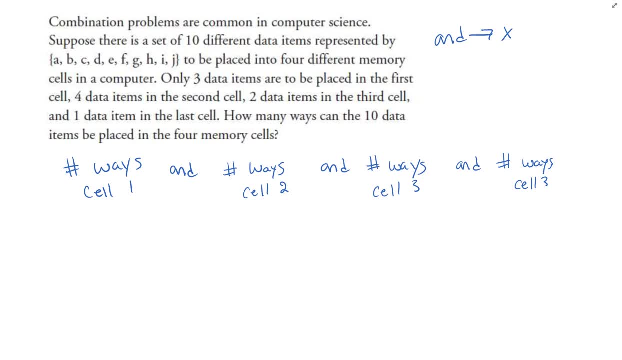 Now, order doesn't matter. It doesn't matter what data item gets played in cell 1, in what order. It just matters that all of the items are in that cell. So this is not going to be a permutation type question, but rather a combination type question. 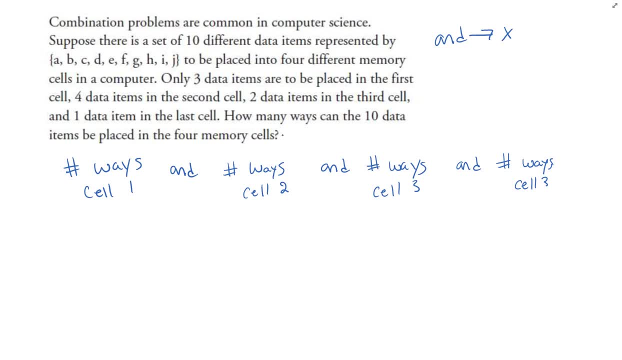 Okay, As long as everybody. Okay, As long as everybody is in that place. So if I look at the first cell, okay, we have 10 different data items to choose from, But if we go back here it says only three data items are to be placed in the first cell. 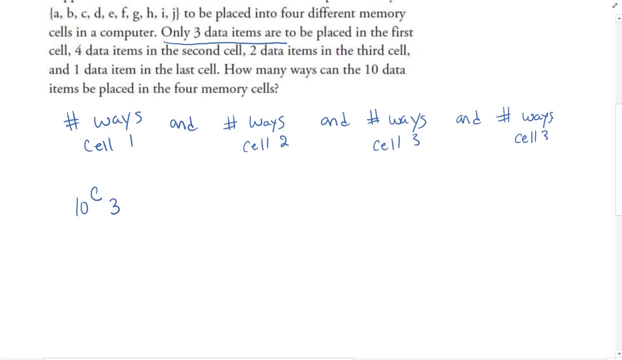 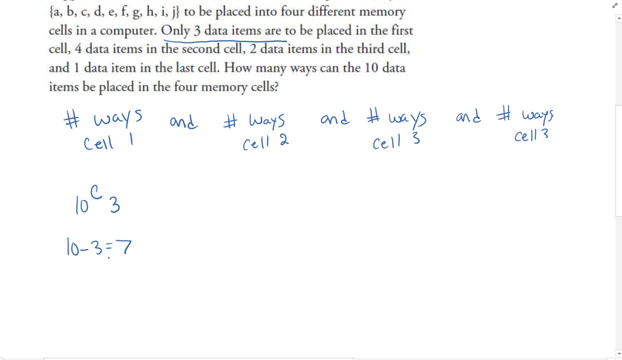 So I can only put three in here. Okay, So those three assume that those three are there. Well, that means I only have seven. So I only have seven left to place, Right, I'm not going to take them back out. 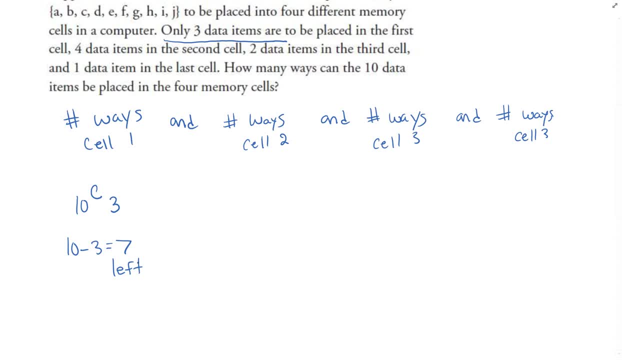 Think about donuts in a donut box. You have 10 donuts to distribute, right? You've taken three of the donuts, put them in that box. You only have seven left to put into box 2,, box 3, and box 4.. 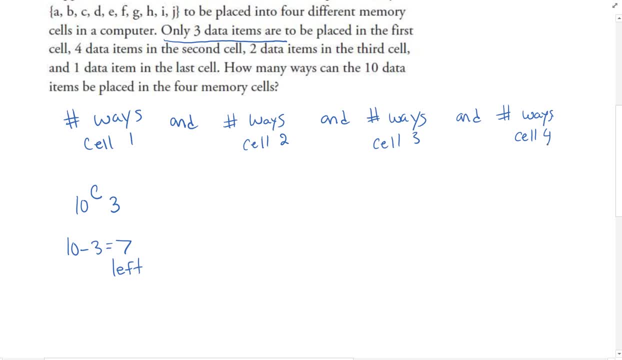 I wrote cell 3 again Four. Okay, So in cell 2, I only have seven left to choose from. But in the second cell it says I get four items can be placed there. Well, those are taken care of now. 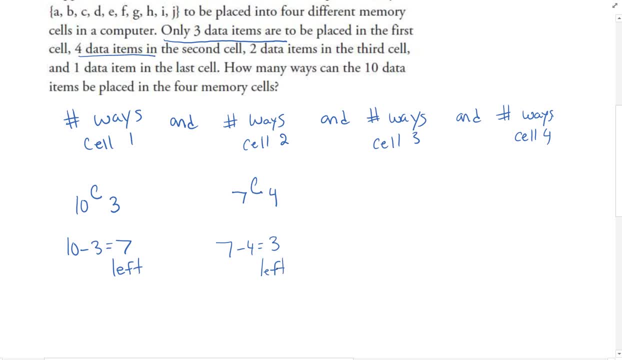 I only have three left, Three left to place in data cell 3. And that would be two items that can be placed in there. So it's 3C2.. Well, 3 minus 2, I'm only left with one. 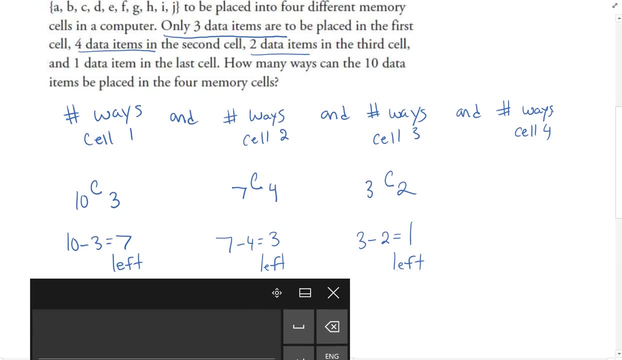 So, finally, in cell 4, it says There's only one data item that can be placed there, And that would be 1C1.. Okay, So we've placed everything: Three in cell 1, four in cell 2,, two in cell 3, and one in cell 1.. 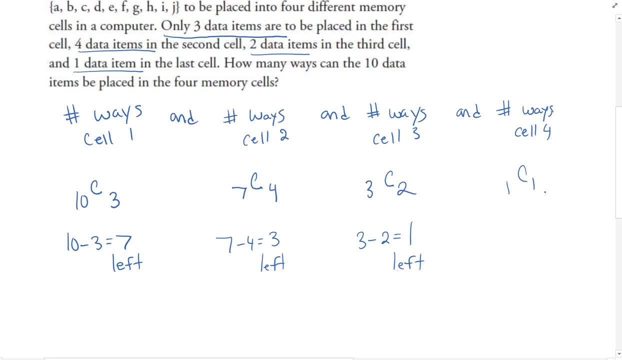 The only thing that's different here, between this and the other cases that we've been looking at and the other examples, is that now How many You have to choose, The number that you choose from is decreasing after you've placed them. 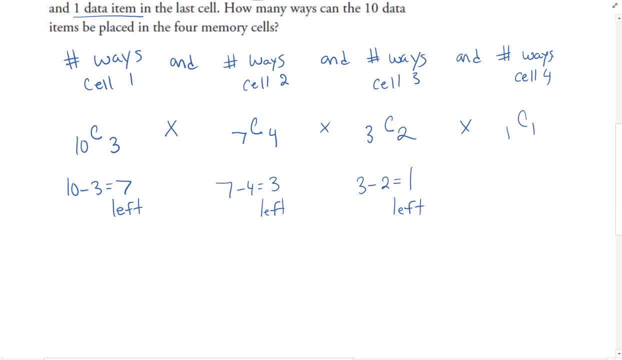 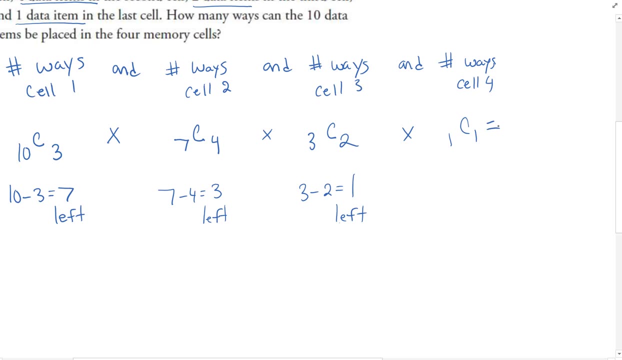 Multiplying those together. Okay, Multiplying all that math together. after you've figured those all out, you end up with Now: you can put it all in your calculator in one shot, or you can do them individually. Double check when you punch that in, then you get the same answer as me as 12,600 ways. 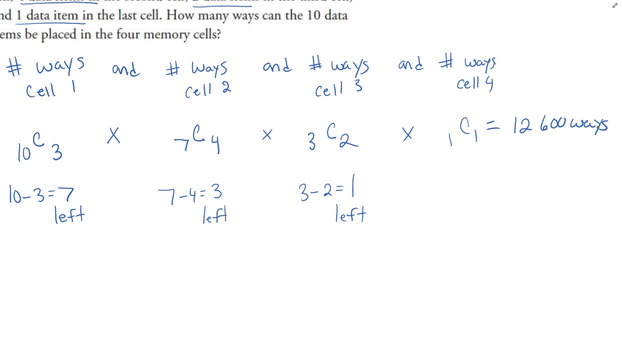 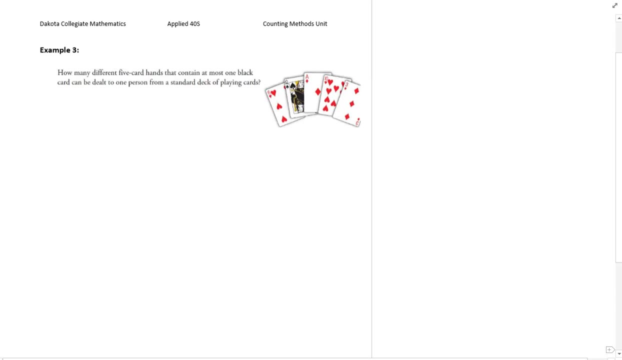 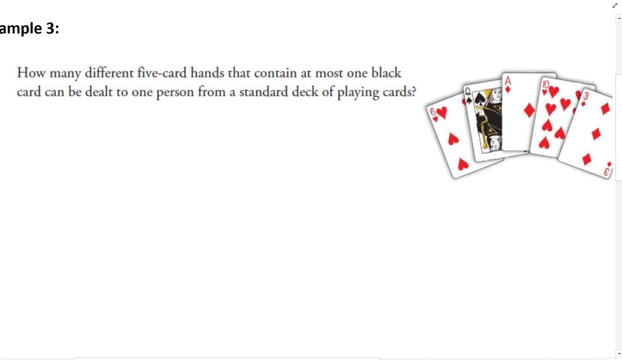 Okay, The last example we're going to look at is example 3, and this has to do with the deck of cards. So it says how many different five-card hands that contain at most one black card can be dealt to one person from the standard deck of playing cards. 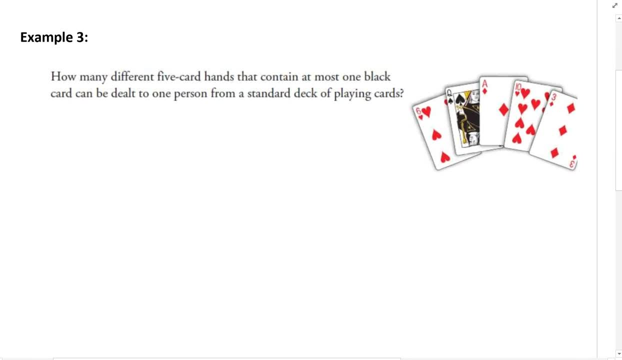 So, again, you need to be familiar with a standard deck of playing cards, Key information here. At most, And when I see it, I'm going to say At most, And when I see it at most that means I have to deal with cases. 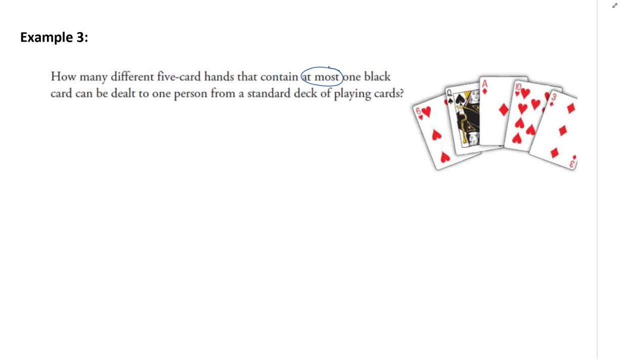 So, at most, one black card means that we can either have one black card or no black cards- Okay, And we're going to have to deal with both of those cases. So let's take a look at case 1.. So if we have one black card and four, 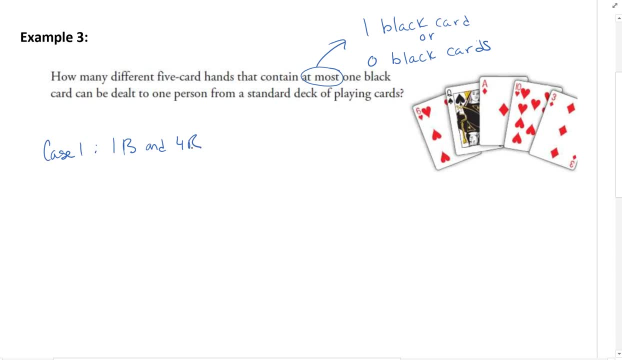 And then we have a deck of cards. We're going to have to deal with both. Okay, So we have a deck of red cards, Right? How many black cards are there in a deck of cards? Twenty-six, But we only want one. 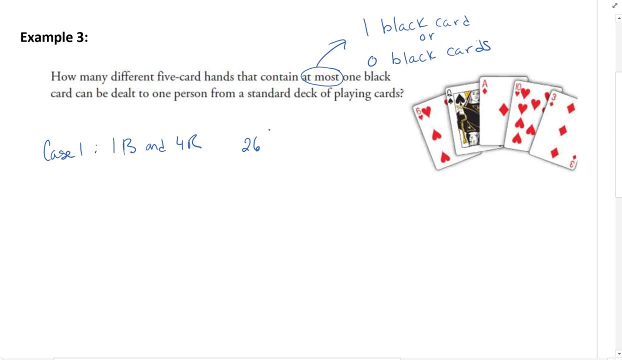 And then, how many red cards do we have in a deck of cards? Twenty-six, And we want four of those, Because it's one black card and four red cards. we're going to multiply that together, Case 2.. Case 3.. 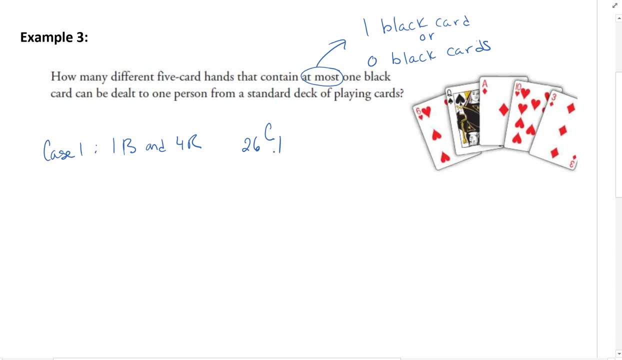 Case 4. Case 5. Case 6. Case 7. Case 8. Case 9. Case 10. Case 11. Case 12. Case, 13. Case, 14. Case, 15. Case 16.. 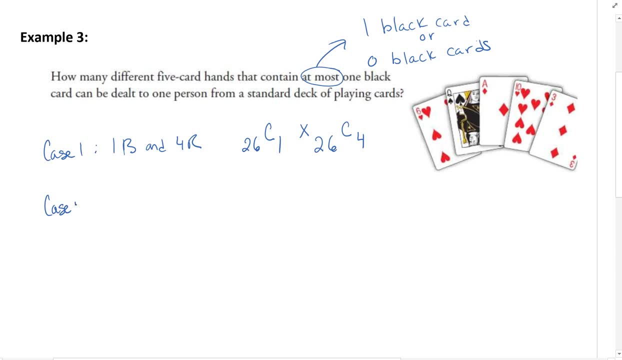 Case 17.. Case 18.. Case 17.. What if there are no black cards and five red cards? Well, that would look the same, but it would be 26C0 times 26C5.. Get those two answers, add them together and you'll get. well, I'll rewrite this: 26C1. 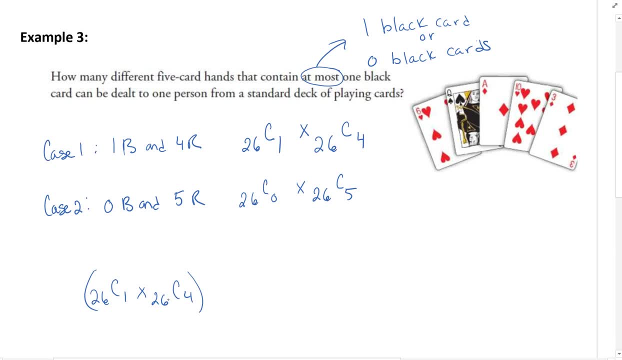 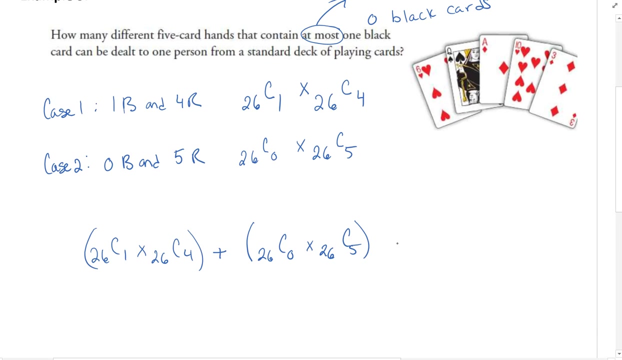 times 26C4.. Do all of that stuff first, because order of operations matters here- 26C0 times 26C5, and then do all that stuff next. Once you get those two answers, add them together and you get a total of 454,480 weeks. 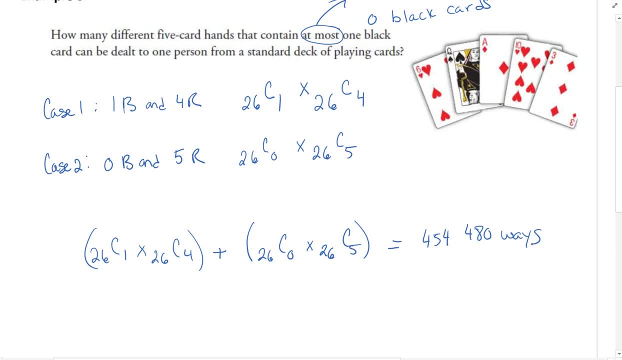 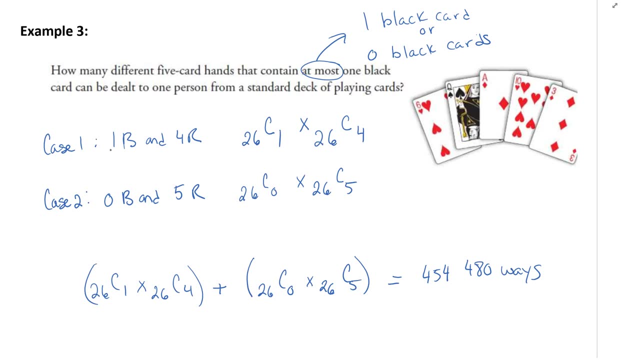 Okay, So again, at least at most- tells you that you're going to get a total of 454,480 weeks. As you were dealing with cases. in each case, one black card and four red cards. we're multiplying. 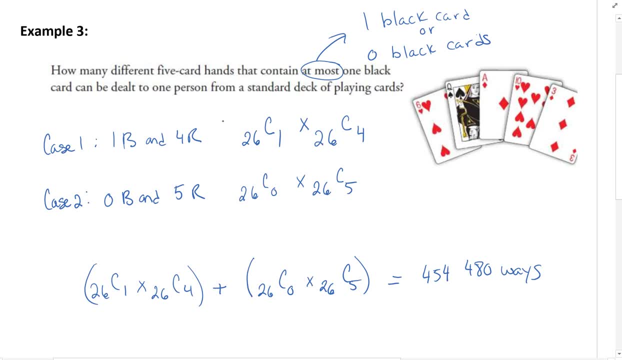 those two combinations together because both have to hold true, and then, looking at each individual case, we're adding them together, because it could be case one or case two, to get a sum. Thanks for joining me today.